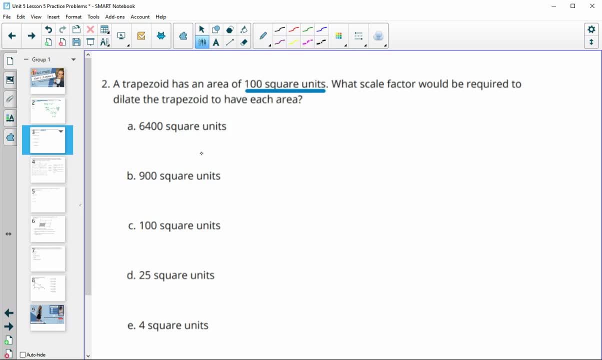 these two areas, you're going to get the k squared. So when we do the new area divided by the original area- so in this case 64 under divided by 100, we're going to get the k squared. So then we'll square root that to get our k value. So new area divided by original area will give us: 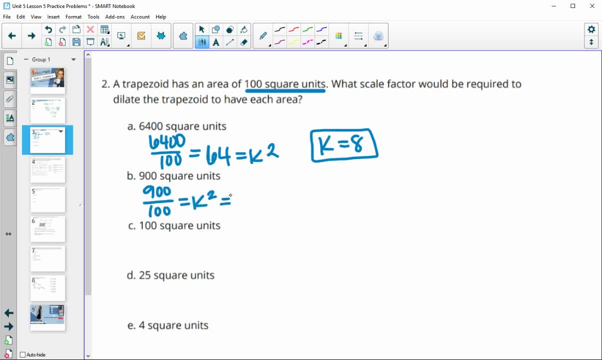 our k squared. Okay, in this case, 900 divided by 100 is 9, square root that and get k equals 3.. So new area is 100, original area is 100. So that didn't change, change in size. So we know that that k value is 1.. New area is 25, original is 100. That's our k. 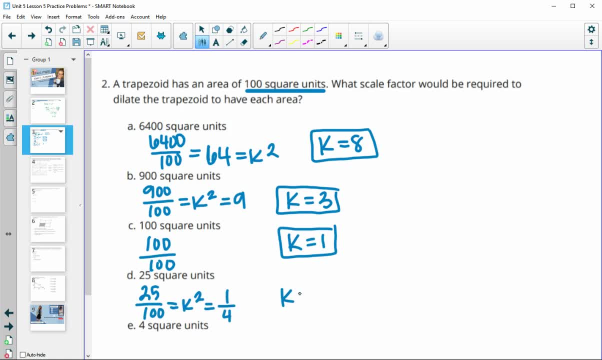 squared, which simplifies to 1, fourth. And so when we square root, this square root of 1 is 1, square root of 4 is 2.. So our k value is 1, half Final one, our new area is 4, our original is 100.. 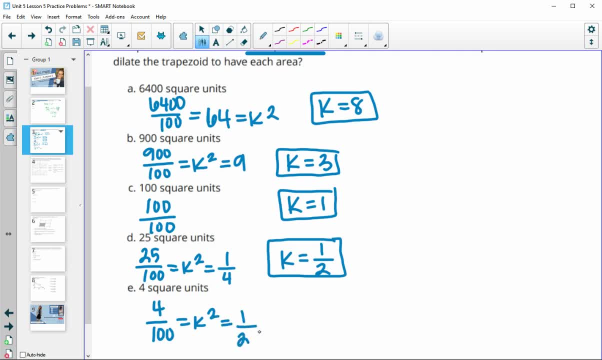 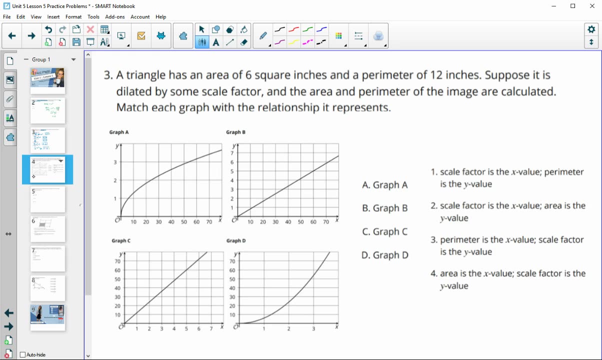 If we simplify that our k squared value is 1 over 25, square root the 1 and you get 1, square root the 25 and you get 5.. Okay, next one: A triangle has an area of 6 inches and a perimeter of 12.. Suppose it's dilated by some. 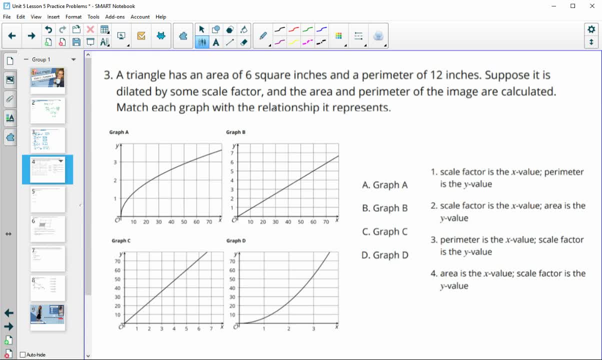 scale factor and the area and perimeter of the image are calculated, Match each graph with the relationship it represents. So we're going to do that, So we're going to do that, So we're going to do that. So, when we're talking perimeter- okay, perimeters are multiplied by just your scale factors. You. 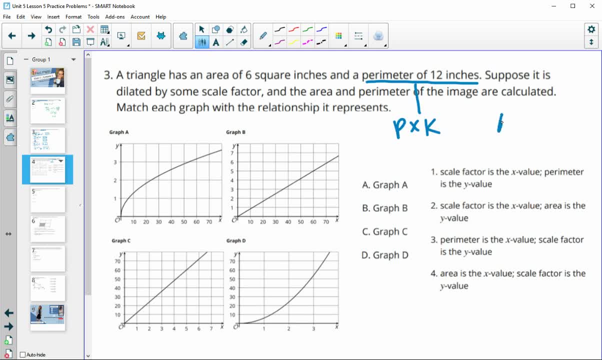 take your original times, just your scale factor And for areas you're multiplying by your scale factor squared. So when we multiply by just the k value, this is going to give us a straight line, And when we're multiplying by k squared, now we're not keeping a linear or direct proportion. 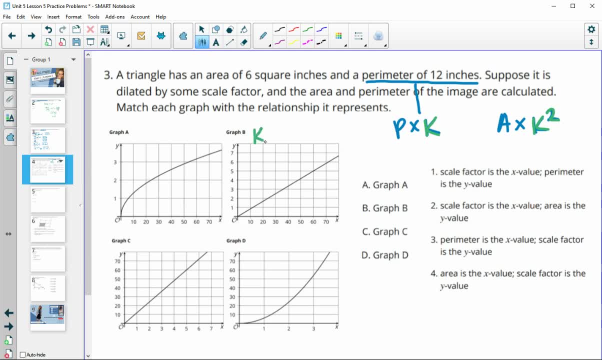 we're going to get some type of curve. So we know that graph B and C are dealing with our k value and A and D are dealing with our k squared or our area. So when we take a look at graph B we see that the larger numbers are kind of 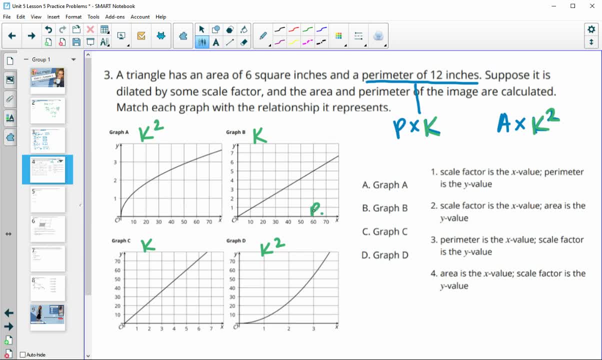 down here at 10,, 20,, 30,, 40.. So those are our perimeters, And one, two, three, four, five, six, seven are our scale factors. And then we see that flipped in graph C, So we see the smaller numbers. 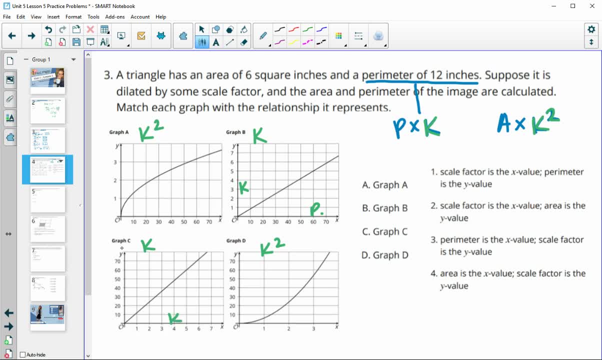 one, two, three, four, So those are our scale factors- And then 10,, 20,, 30,, 40 representing those perimeters. And so let's take a look here. So number one says the scale factor is the x value. 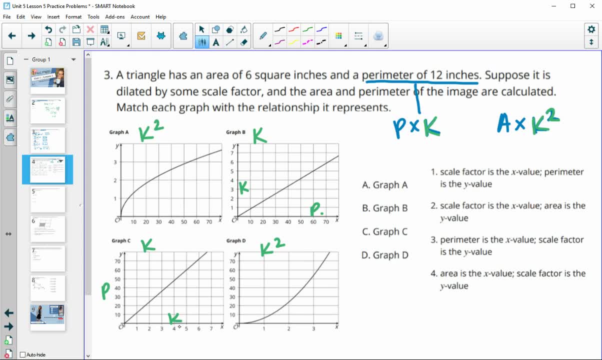 the perimeter is the y value. So scale factor is the x value, perimeter is the y value. this is graph C, So the other one dealing with perimeter is graph B, And so that says perimeter is the x value which we see and scale. 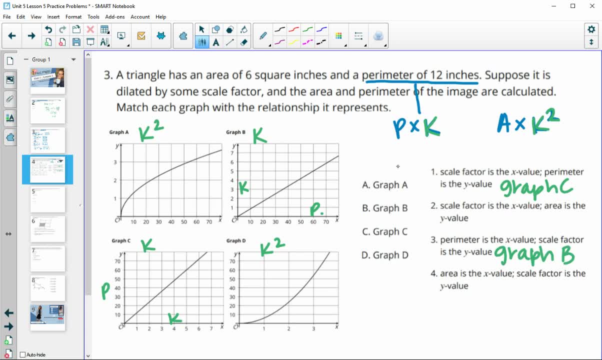 factor is the y value. All right, then, in the next ones we're dealing with the area. So when you see again, we see this: one, two, three on this scale. this is our k squared, or our scale. well, not our k squared. 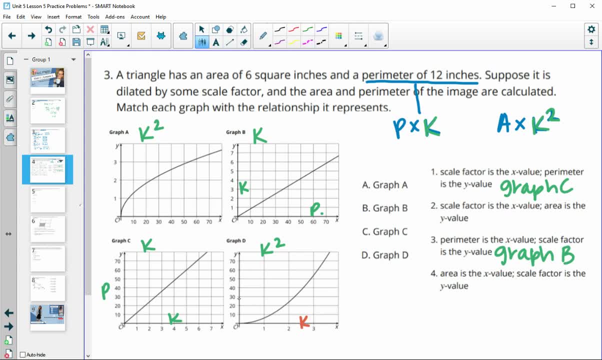 but this is our k, our scale factor, and then our areas, And where this one has the x value as the areas and the y value as the scale factor. So number two here says the scale factor is the x value. So which one of these have the scale factor as the x value? and that's graph D, So that 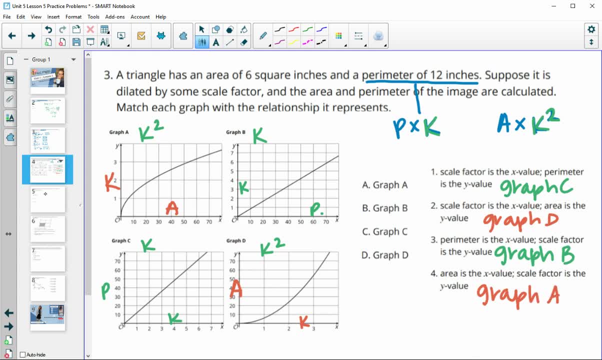 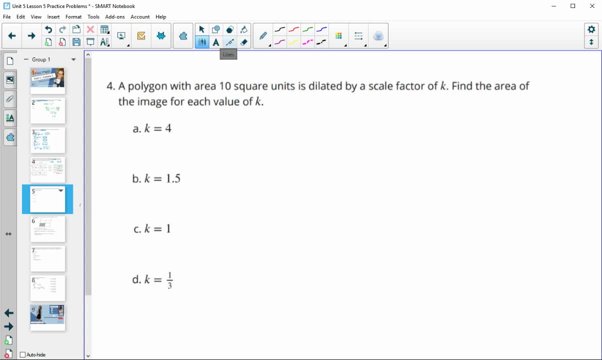 leaves graph A for number four. Number four polygon has an area of 10 square units, is dilated by: okay, so area of 10 square units is dilated by a scale factor of k. find the area of the new image. So they're giving us our k value in each of these problems. So remember, we for our. 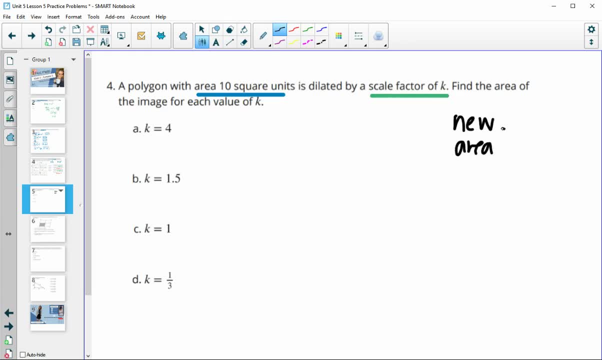 new area. we need to take our original and we need to multiply it by our k squared, Since there's two dimensions and finding area. we're going to dilate. We're going to end up with this k factor in there twice. So we're going to take our original area in each of these problems, which is 10.. 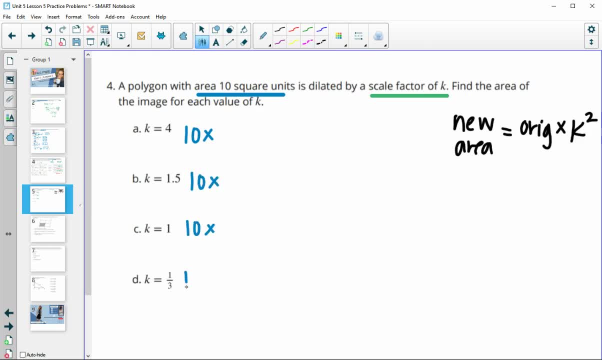 Okay, so we're going to do 10 times the scale factor squared, So I'm just going to get this written for all of them. Then we're going to take and multiply times the scale factor squared, So 4 squared, 1.5 squared, 1 squared, 1 third squared, and then this will get us our 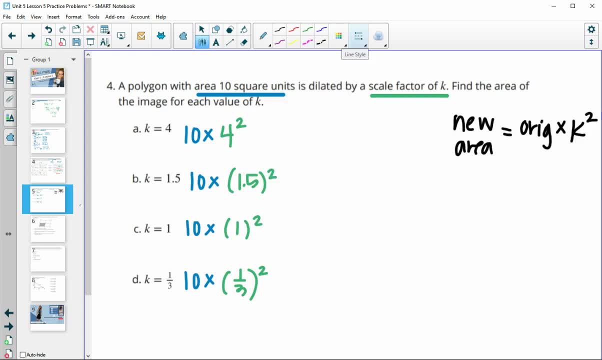 new area. So 10 times 4 squared, so 10 times 16, is going to give us 160 units squared for our new area. Um 10 times 1.5 squared is going to give us 22.5 units squared for the new area here. 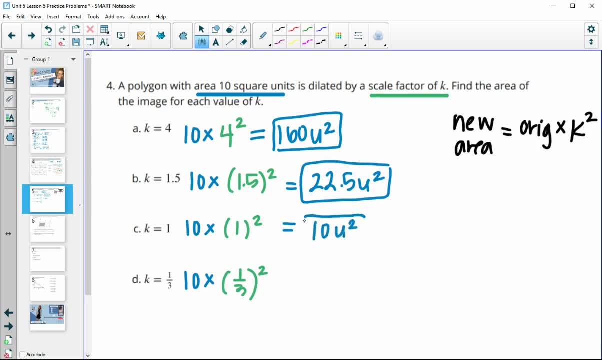 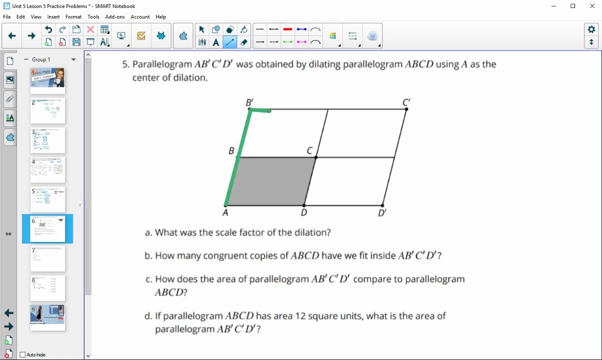 10 times 1 squared stays 10, so just 10 units squared. That one didn't change in size. And then 10 times 1, third squared, here is 1.11 units squared. Number five: parallelogram: A, prime, B prime, C prime, D prime. So this larger. 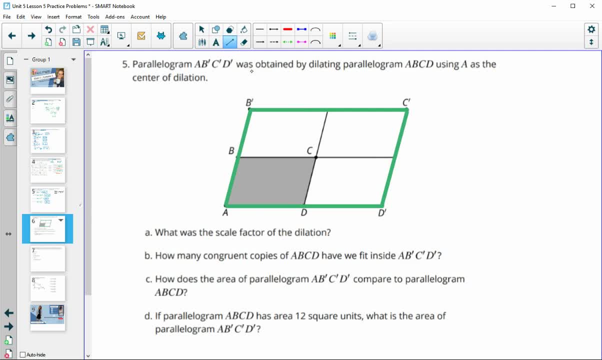 parallelogram here, um is, was obtained by dilating um parallelogram A, B, C, D, using A as the center of dilation. So taking this shaded parallelogram and dilating it, keeping point A kind of the same, since that's the center of dilation. 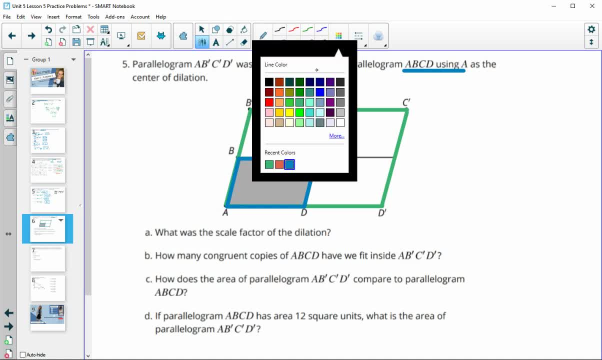 What is the center of dilation? What is the scale factor? So remember, scale factor is um kind of how much you multiplied each length by. So we see, to go from A, B to A prime, B, prime, Okay, that's double the length. 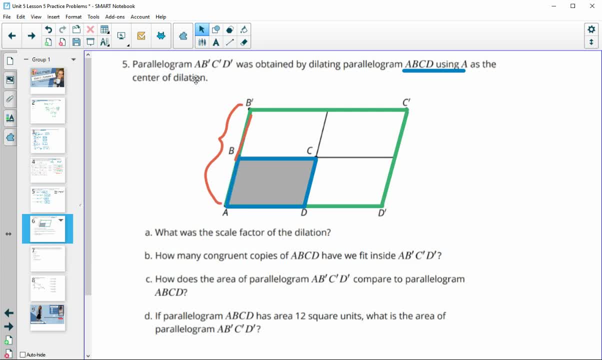 So this would fit in there twice. Okay, so that's scale factor. Each side length is two times bigger. How many congruent copies of the original parallelogram fit inside of the original parallelogram? So we see, here's one, two, three, four parallelograms fit in there. 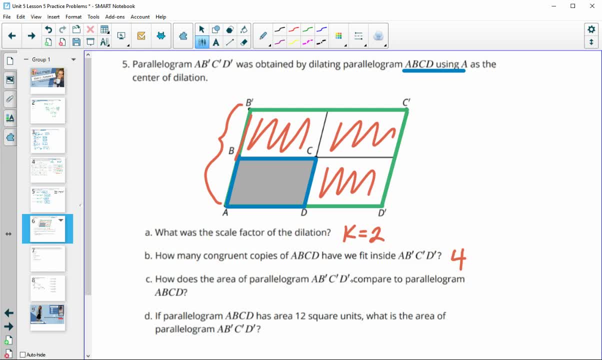 So how does the area of parallelogram A, prime, B, prime, C, prime, D prime compare to parallelogram A, B, C, D? So this green one is four times bigger than the original, since four of the original fit into the green one. 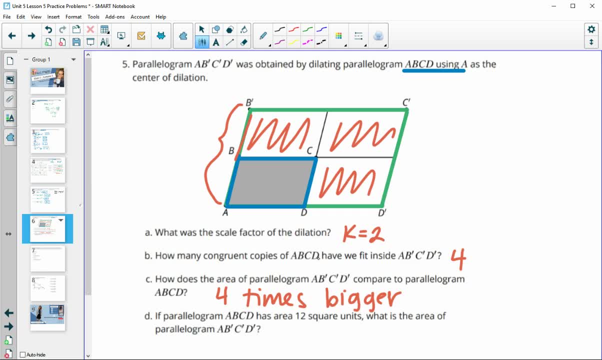 So parallelogram A, B, C D: how many congruent copies of the original parallelogram A, B, C, D has an area of 12 square units. So if this one is 12 square units, what's the area of the larger? 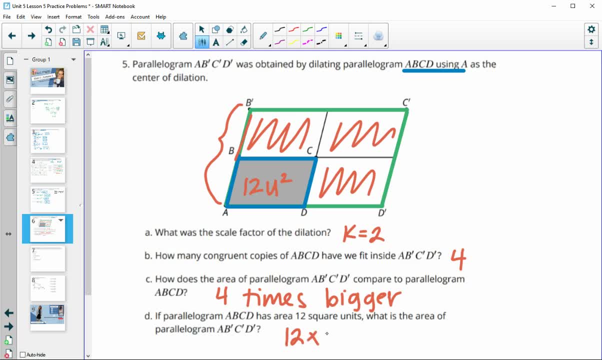 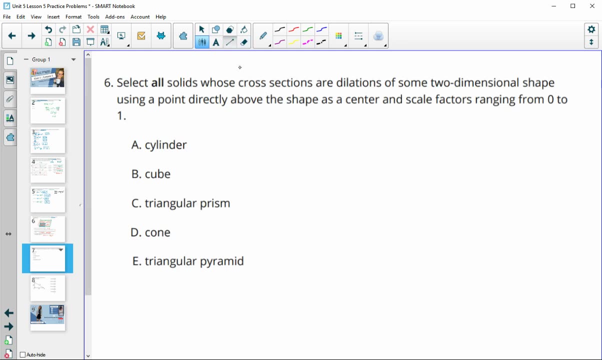 one. So we know that that 12 square unit parallelogram fits into the larger one four times. So then the larger one would be 48 units squared Number six: select all solids whose cross sections are dilations of some two-dimensional shape, using: 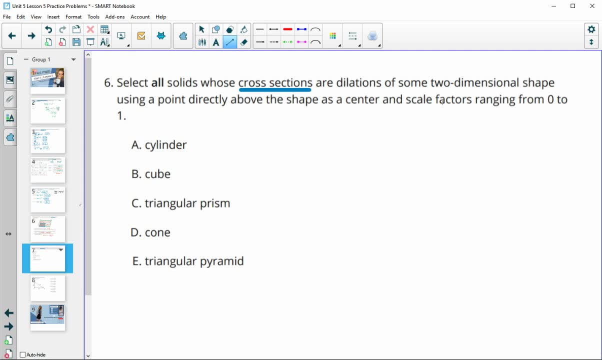 a point directly above the solid. So we see, here's one, two, three, four parallelograms fit into the of the shape as the center and scale factors ranging from zero to one. So this means that it's getting smaller as we go because you've got your point of dilation, you've got whatever's. 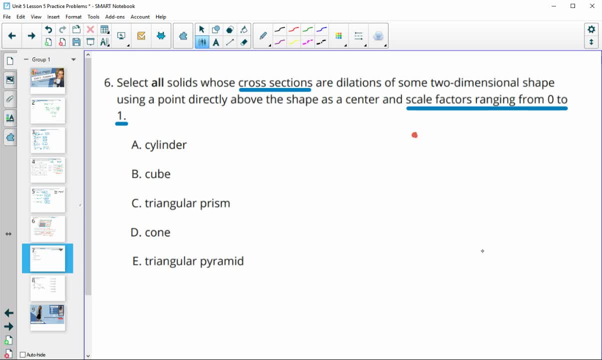 happening like, whatever shape it is, the original cross section would be the scale factor of one, and then all the way up to a scale factor of zero, going to a point, And so then this is just going to keep getting smaller and smaller as we go. So this is going to keep getting smaller and 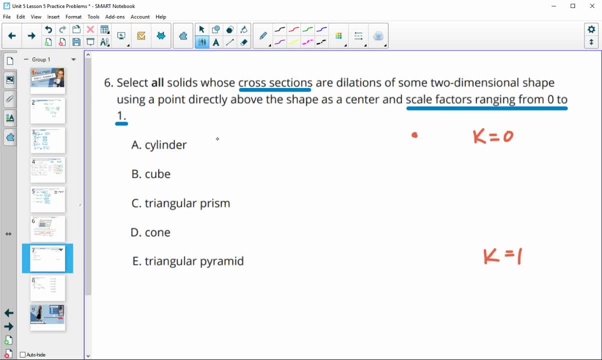 smaller as you go. So a cylinder does not get smaller as we go. the cross sections stay the same all the way up. Okay, so that's not good. A cube- same thing. it's got a bunch of squares that stay the same size from top to bottom. Okay, so those cross sections don't change. Triangular.